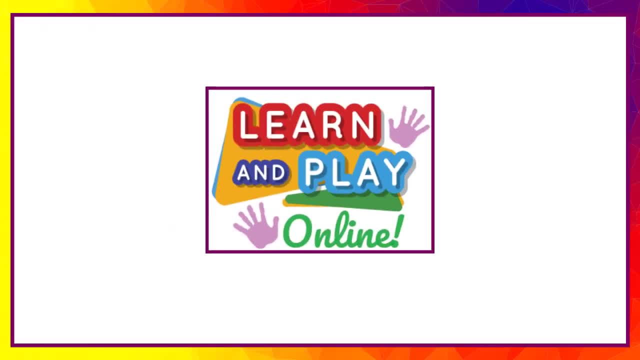 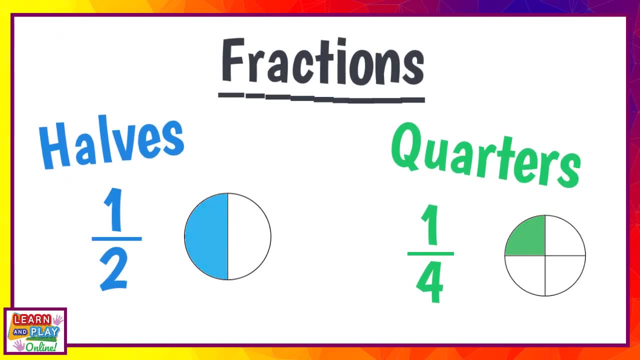 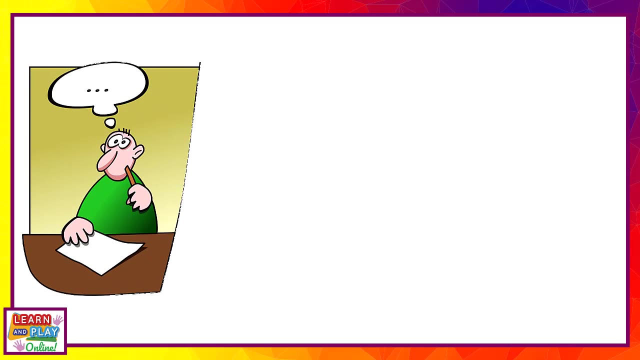 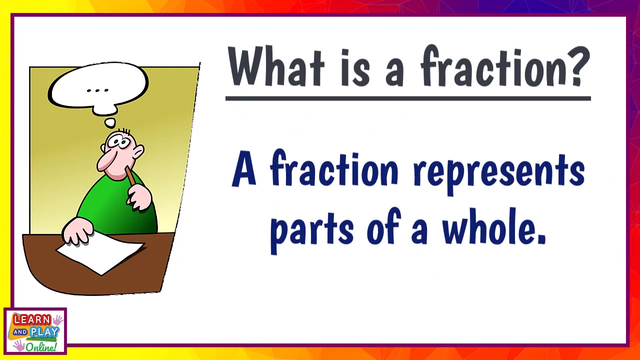 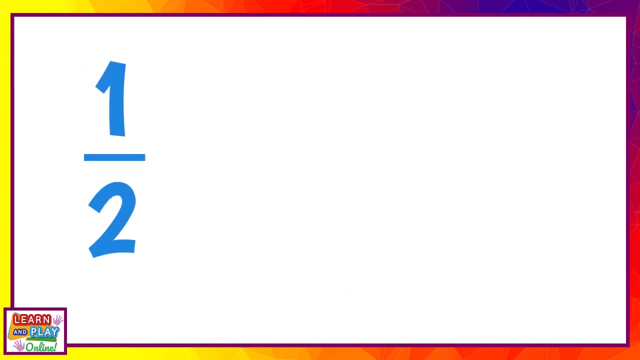 Learn and play online. Today, we are going to learn about fractions, halves and quarters. You might be wondering: what is a fraction? Well, a fraction represents parts of a whole. This is an example of what a fraction looks like. The number at the top is called the numerator. 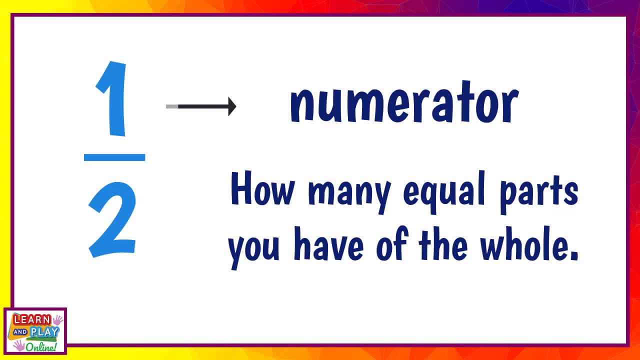 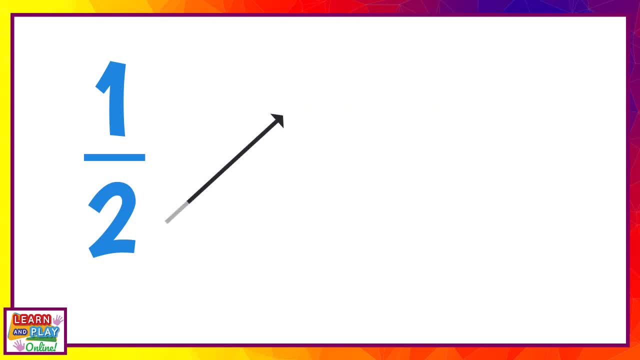 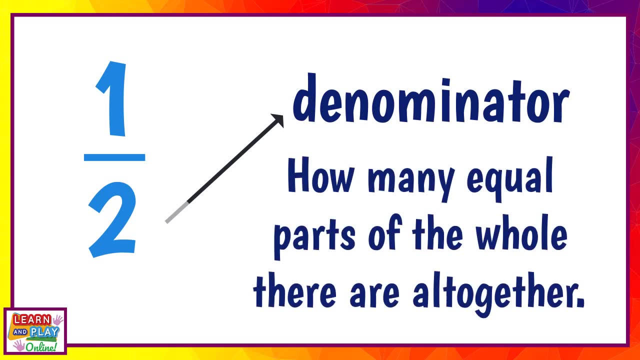 The numerator tells us how many equal parts you have of the whole. The number at the bottom is called the denominator. The denominator tells you how many equal parts of the whole there are altogether. Now let's go through some examples so we can have a better understanding. 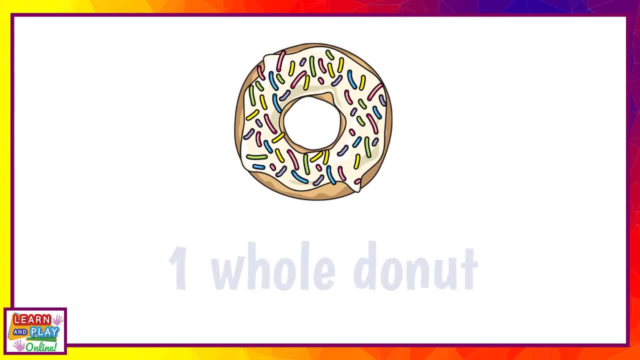 Here we have one whole doughnut. If I wanted to share the doughnut with someone, I would have to cut it into equal parts and make it fair. If I cut my doughnut like this, I'll have one small piece and one big piece. 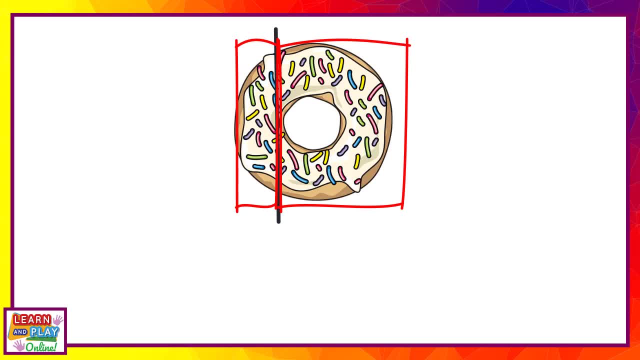 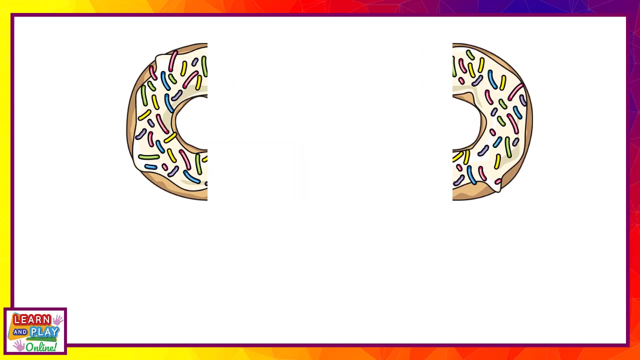 That means they are not equal parts. So let's try that again. This time I cut the doughnut into two equal parts because they are the same size. When you have cut something and have two equal pieces, that means you have cut it into half. 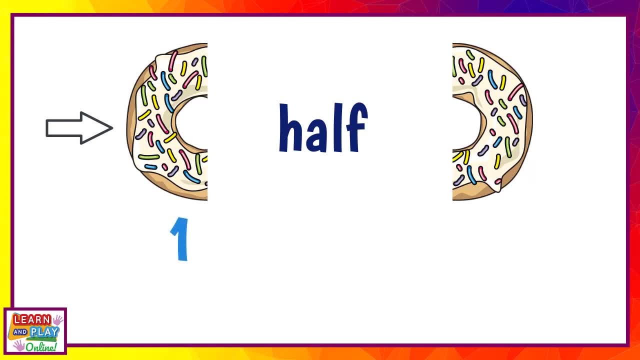 On this side I have one piece of the doughnut, which is why the numerator is one, But altogether there are two pieces, and that's why the denominator is two. That's the same for this piece as well. Over here we have one piece of the doughnut. 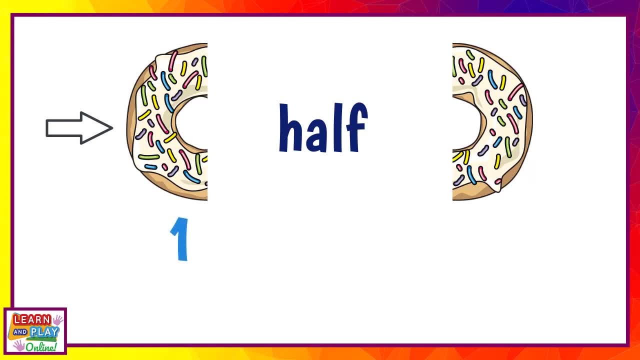 On this side I have one piece of the doughnut, which is why the numerator is one, But altogether there are two pieces, and that's why the denominator is two. That's the same for this piece as well. Over here we have one piece of the doughnut. 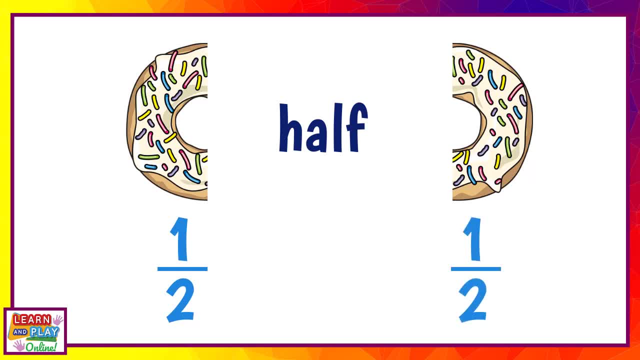 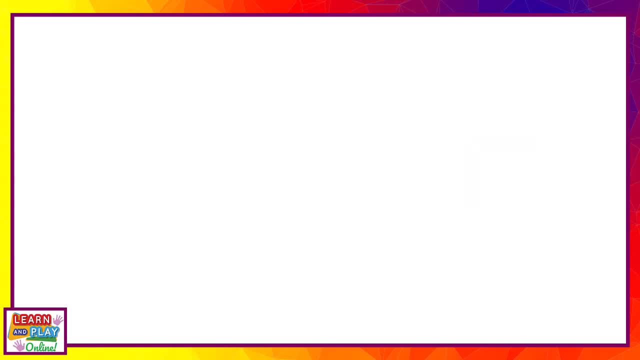 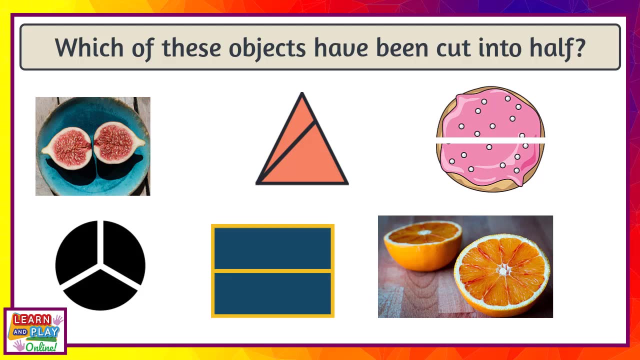 but there are two pieces altogether. Each piece shows half of the doughnut. Have a look at these pictures. Which of these objects have been cut into half? Remember, an object has been cut into half. if there are two equal pieces, You can pause the video to discuss it with someone. 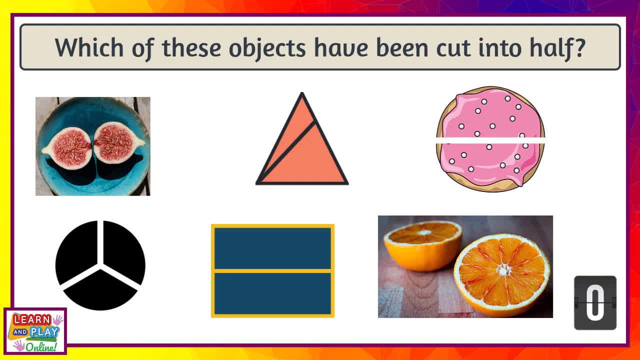 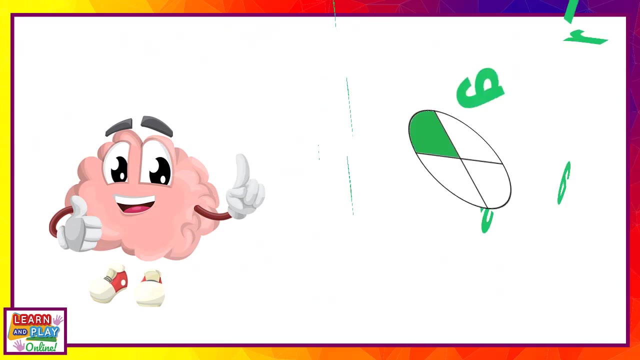 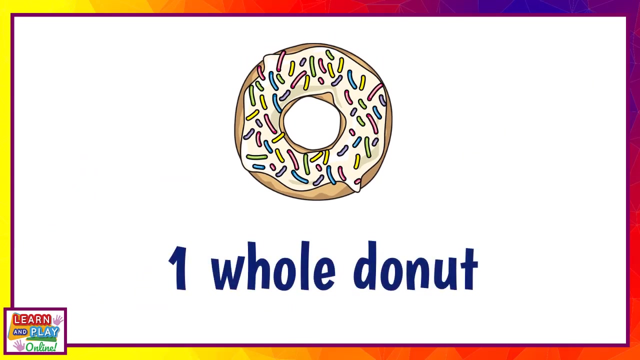 We are now going to show you the answers. The objects that have been circled have been cut into half because they all have two equal parts. Let's now move on and learn about quarters. We are going to use one whole doughnut again. 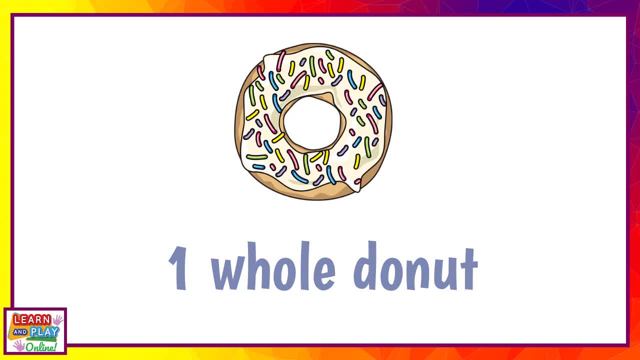 But this time, to make quarters we need to make four equal parts. First we'll cut the doughnut into half. Now we have two equal parts. To make quarters we need four equal parts. So let's cut it in half again. 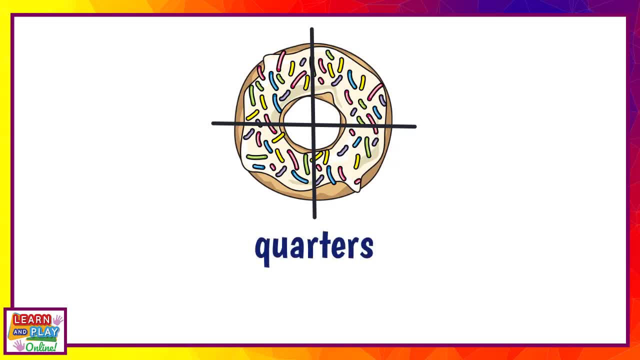 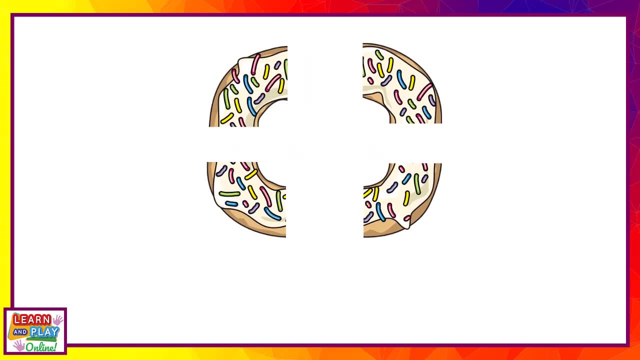 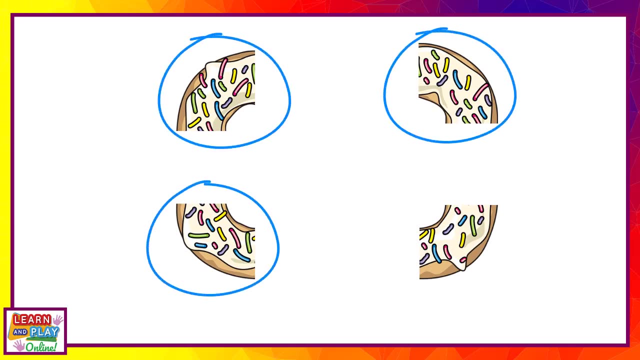 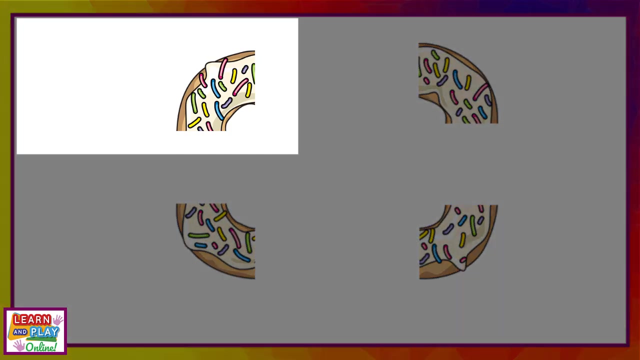 The doughnut has now been cut into quarters, because there are four equal parts. Let's count them together: One, two, three and four. Let's look at this piece on its own. Here we have just one piece, which is why the numerator is one. 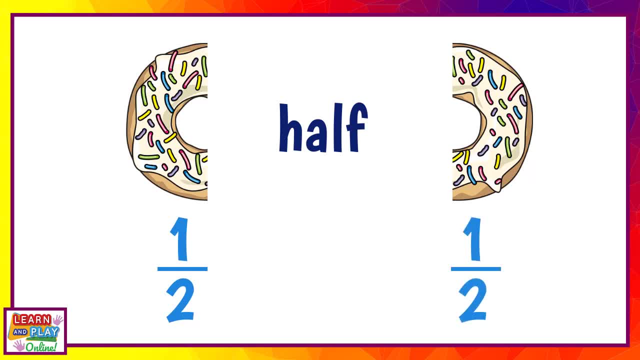 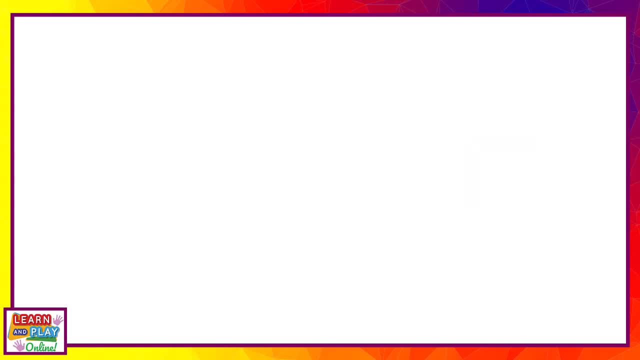 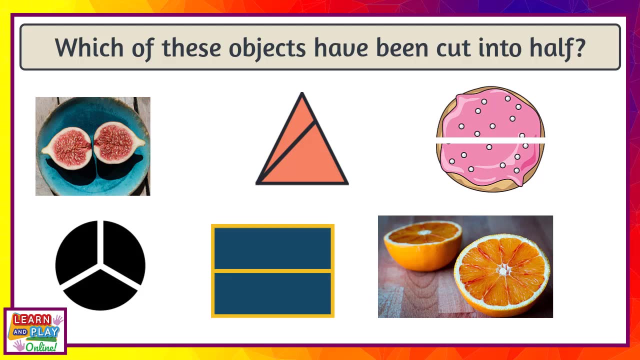 but there are two pieces altogether. Each piece shows half of the doughnut. Have a look at these pictures. Which of these objects have been cut into half? Remember, an object has been cut into half. if there are two equal pieces, You can pause the video to discuss it with someone. 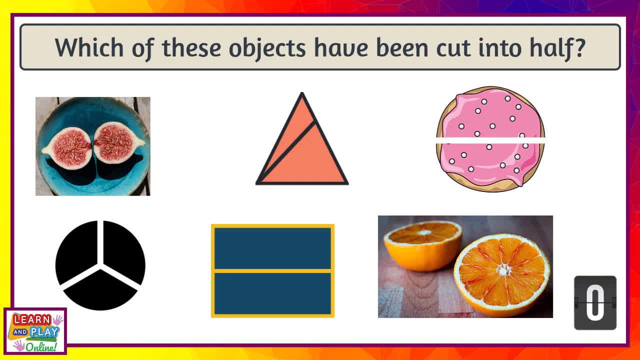 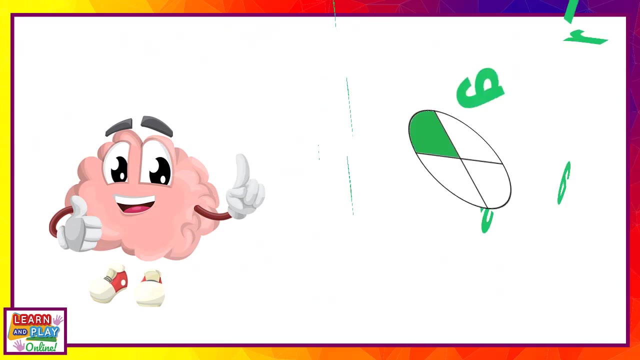 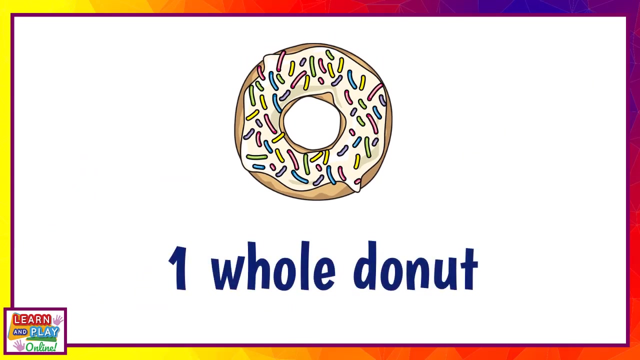 We are now going to show you the answers. The objects that have been circled have been cut into half because they all have two equal parts. Let's now move on and learn about quarters. We are going to use one whole doughnut again. 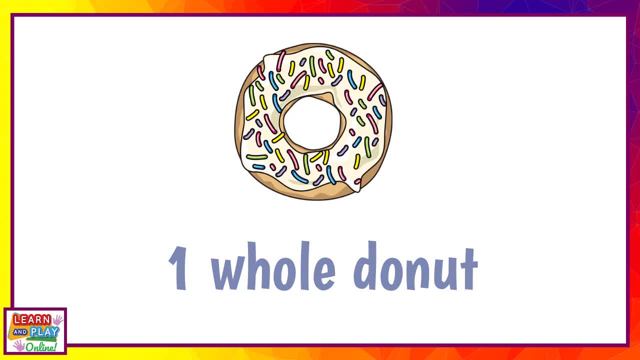 But this time, to make quarters we need to make four equal parts. First we'll cut the doughnut into half. Now we have two equal parts. To make quarters we need four equal parts. So let's cut it in half again. 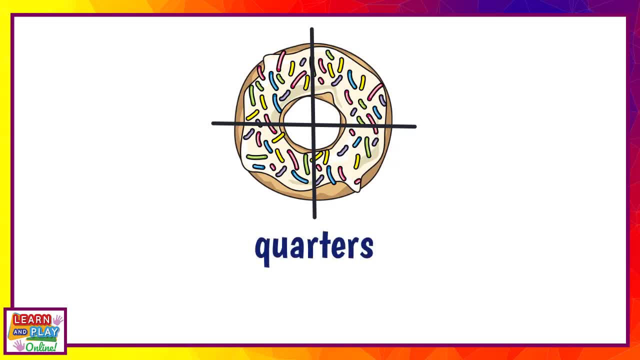 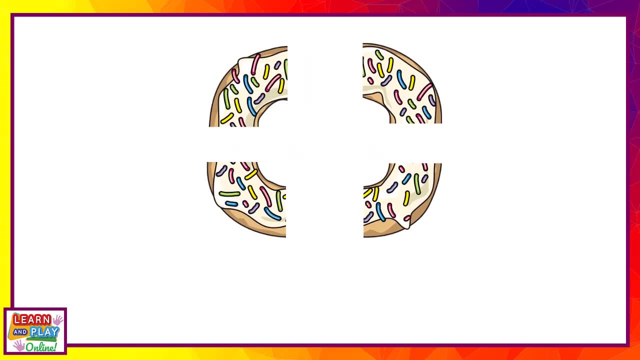 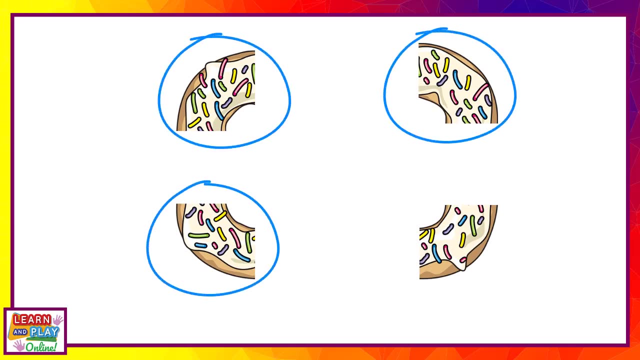 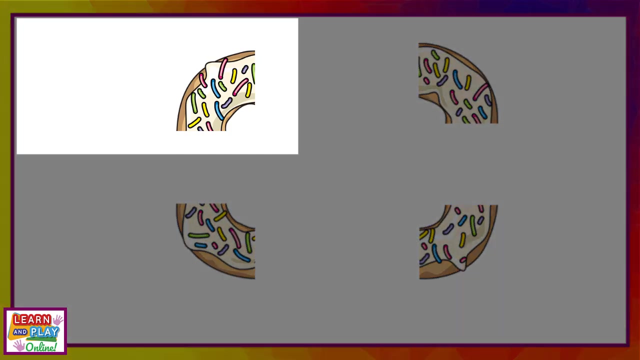 The doughnut has now been cut into quarters, because there are four equal parts. Let's count them together: One, two, three and four. Let's look at this piece on its own. Here we have just one piece, which is why the numerator is one. 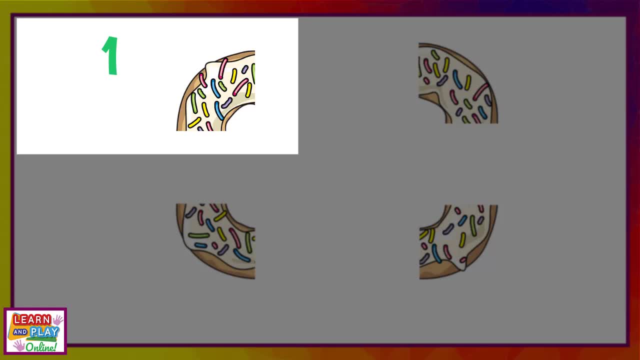 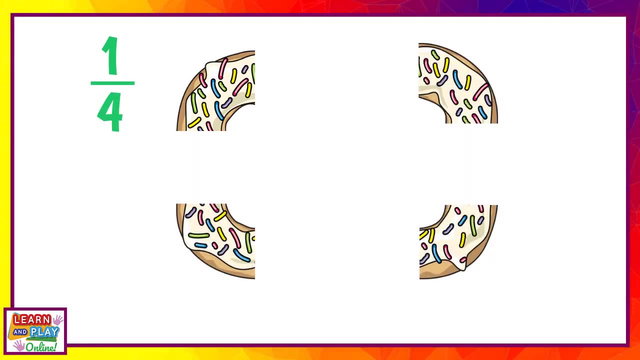 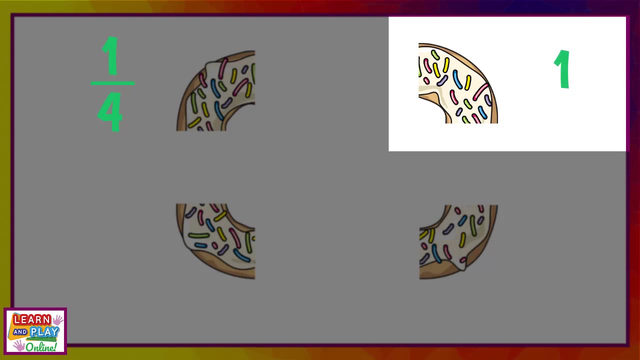 But altogether there were four pieces, which is why the denominator is four. That is the same for this piece as well. This is one piece of the doughnut, which is why the numerator is one, But there are four pieces altogether, which is why the denominator is four.